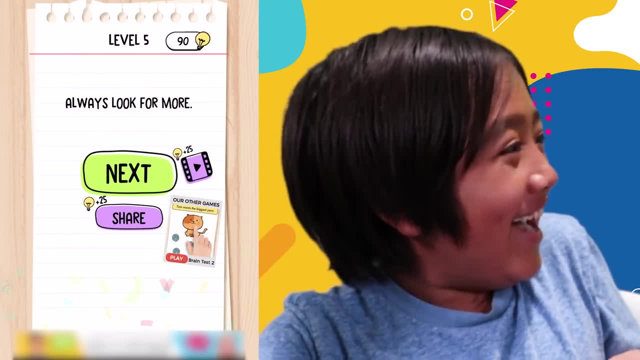 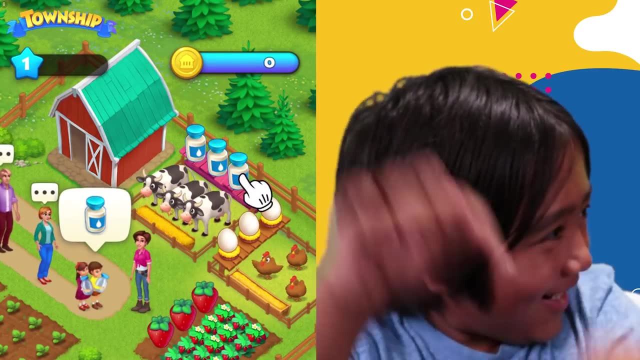 one, I got eleven. How is it eleven? I don't know What. Always look for more. Oh what, I was just pressing the higher button and then submit. Okay, maybe my IQ is not very high. I don't get it. 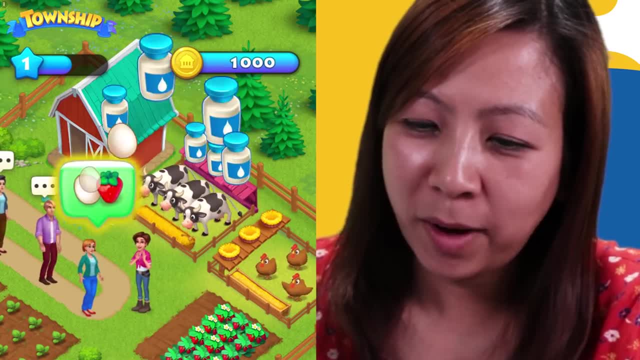 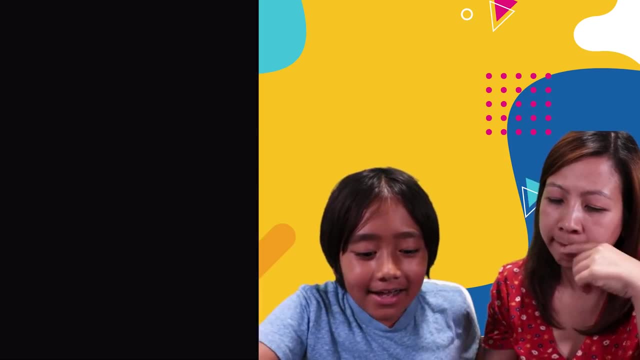 Wow, Is there a way I can just pay for no ads? Oh, I can remove ads. Yay, Thank you. Sorry, guys, Gotta move the ads. You gotta move the ads. No ads. Oh, no, Guys, I thought we removed the ads. 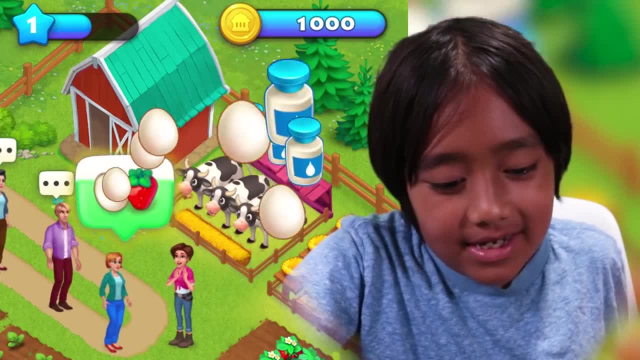 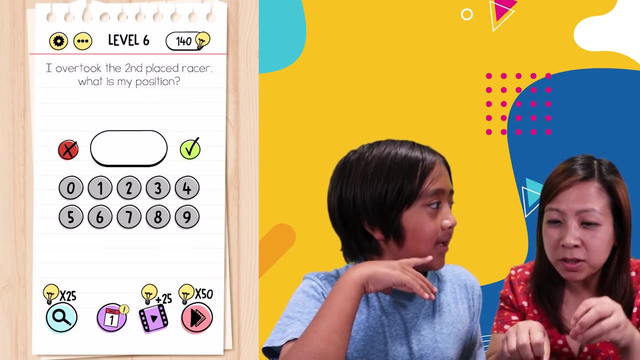 I think I pressed on something. Dude, You get egged. I overtook the second place racer. What is my position? It's not one Second place, Because if you overtook the second place, then you're in second place. 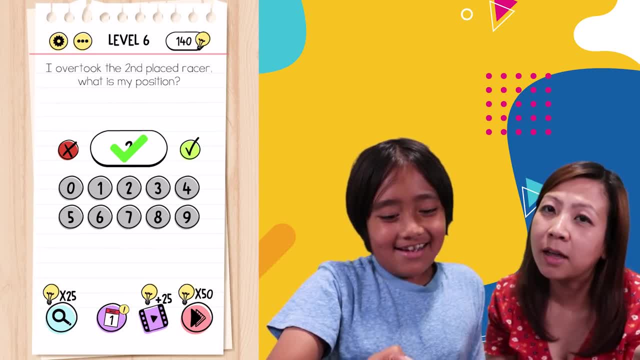 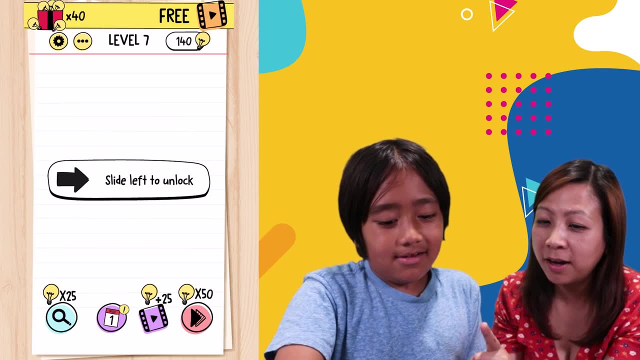 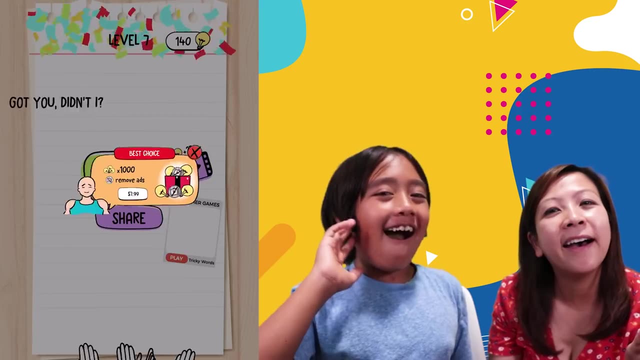 Right. Yeah, I'm smarter than I, look guys. Okay, So good, Slide left, Not right, Slide left. Be careful, It doesn't work. How do you slide left? Ahhh, That's why you need me on your team. 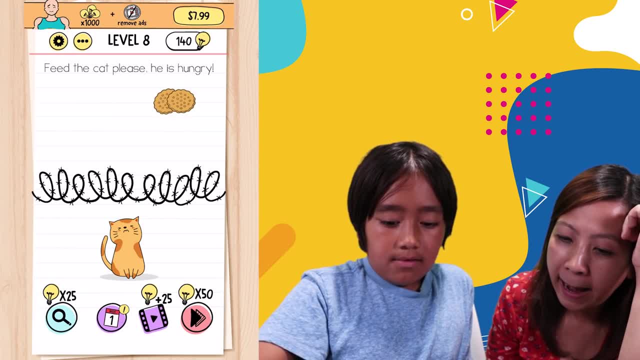 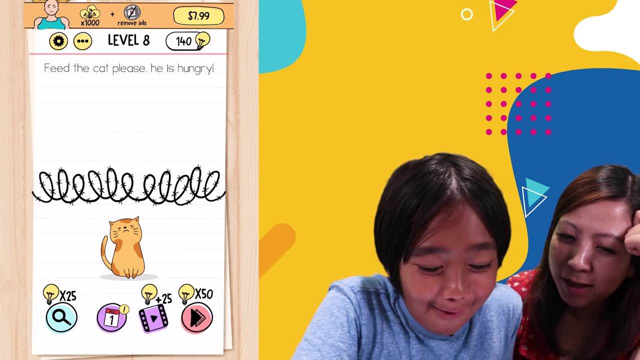 Feed the cat please. He is hungry. How do we do that? There's little spikes in the way, guys. Oh no, Oh no, Oh no, We lost the cookie. Can we reset? Okay, How do we? 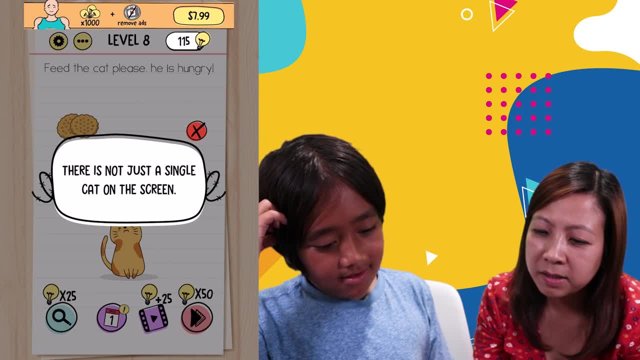 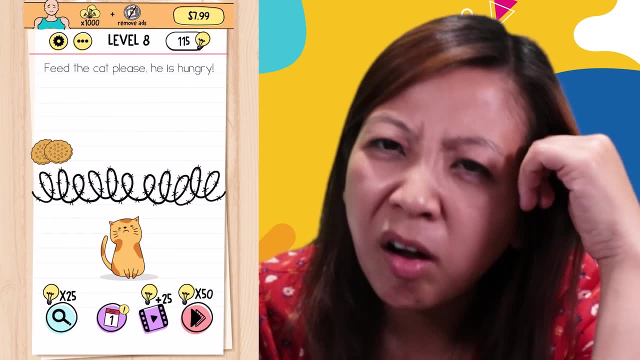 feed the cat. Here we have some hints. Okay, There is not just a single cat on the screen. What, What cat? I don't see any other cat. Where's the other cat? This one is hard Put it like everywhere. 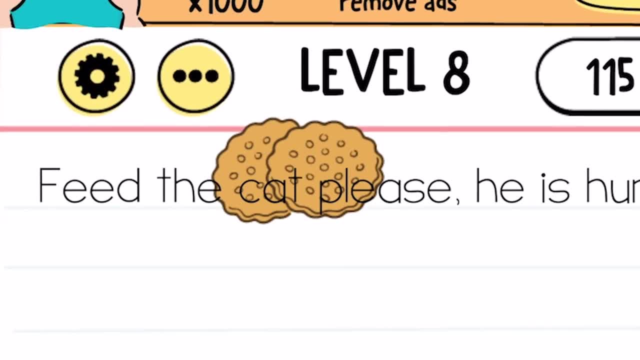 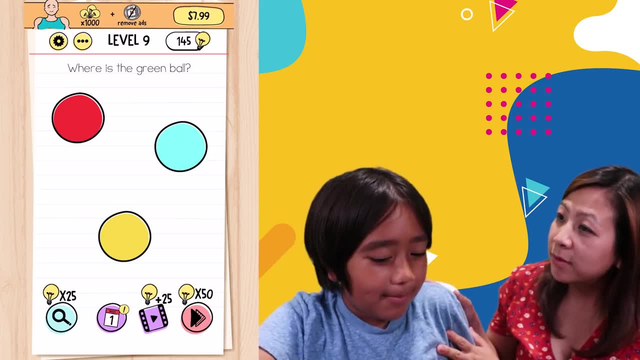 What, What Was there? a cat, The cat, Oh, feed the cat. Really, The word cat is also cat. Where is the green ball? Oh, The green ball. Yeah, We mixed the two colors together. Did you guys get that? 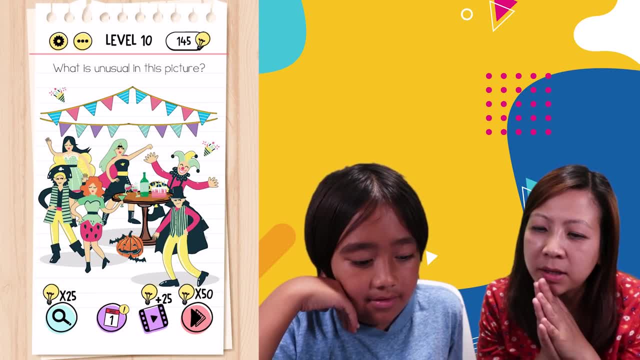 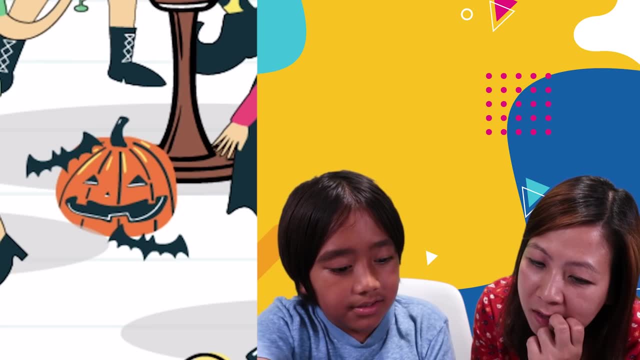 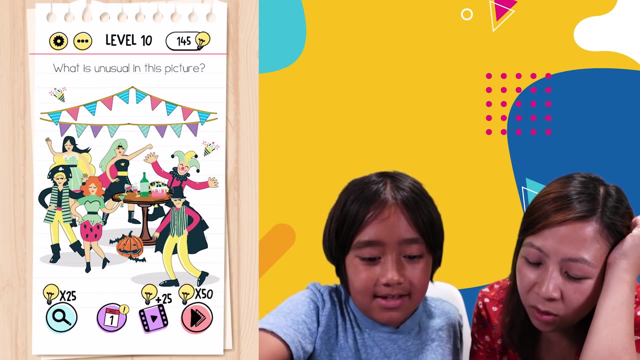 Two colors together, Color math. Who is usually in this picture? What is unusual? Oh, what is unusual in this picture? This The pumpkin. Why Just wait Party. What is unusual? The word unusual, Huh. 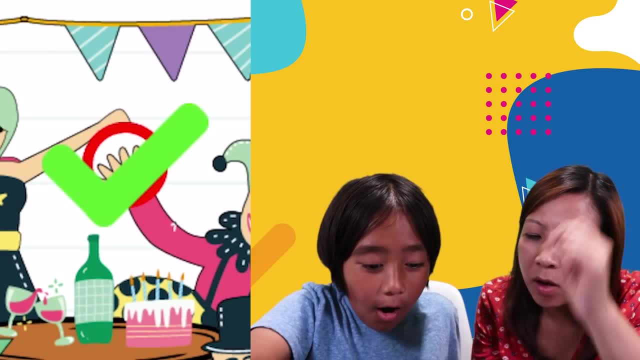 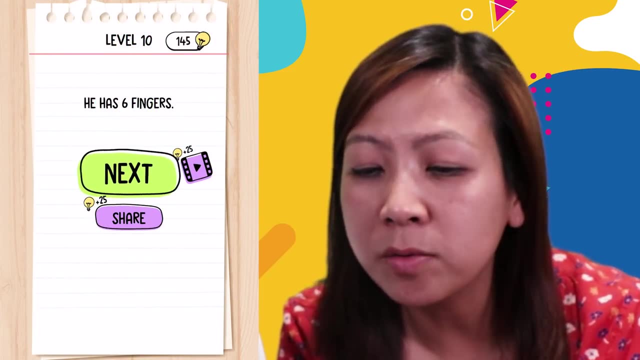 What is unusual? What's different about this picture, guys? I think we need a hint. The hand- Why is the hand unusual? How is that? The fingers? Oh, March, February, May, Which one is longest? Ah wait. 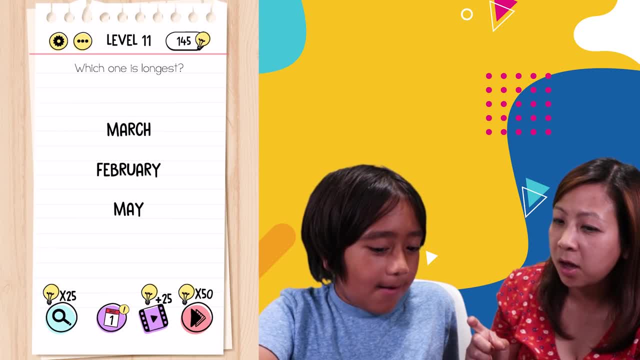 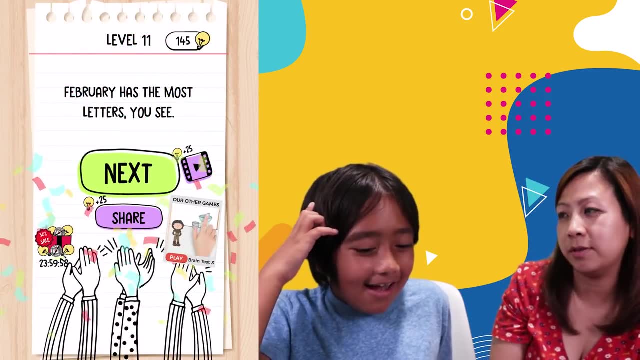 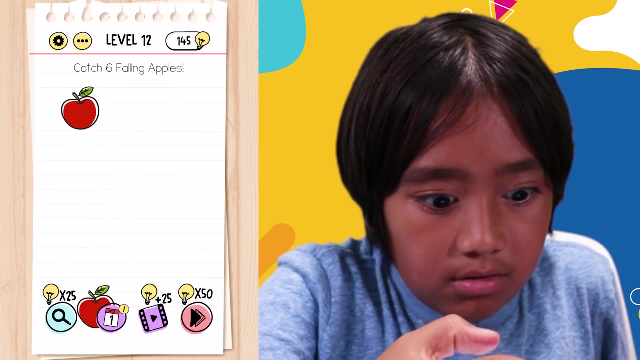 Is the word or the days in the month Which one is longest- March, May, February- Because the word February had more letters. Oh, I thought like: uh, Catch five falling apples, One That's not falling, Those aren't falling. 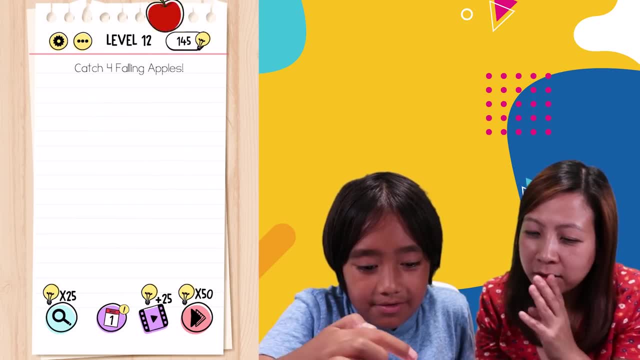 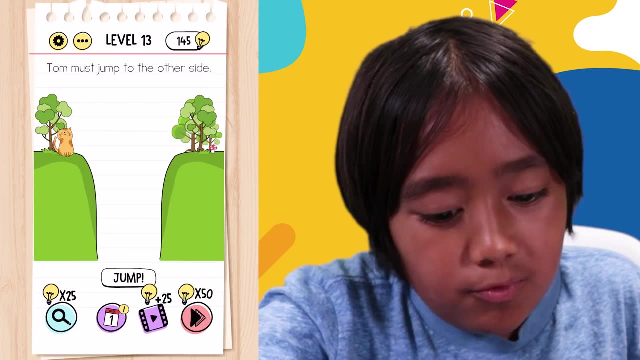 Dot, There you go. Oh, that's not falling. Dot, dot, dot, Yay, Yay, yay, yay, yay, yay. Tom must jump to the other side. Who's Tom? How do we know that it's a cat? 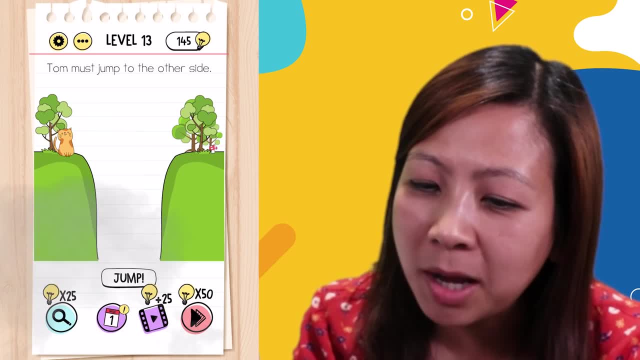 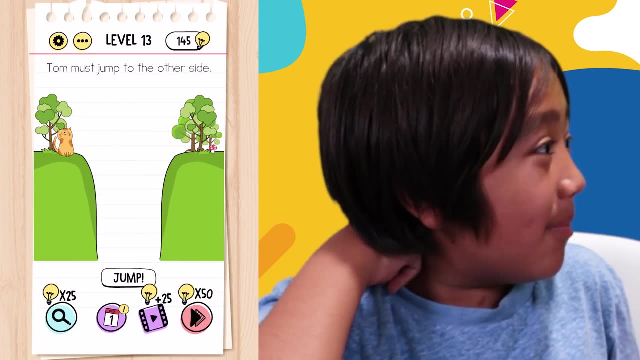 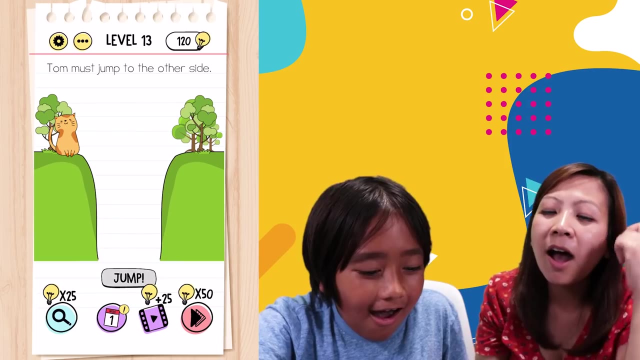 We don't even know. Double jump, Charge jump. Maybe that's not even Tom, But it's making him jump. We need a hint. Try the mushroom. Oh, We feed the mushroom. We feed the mushroom to the cat and then it'll jump higher. 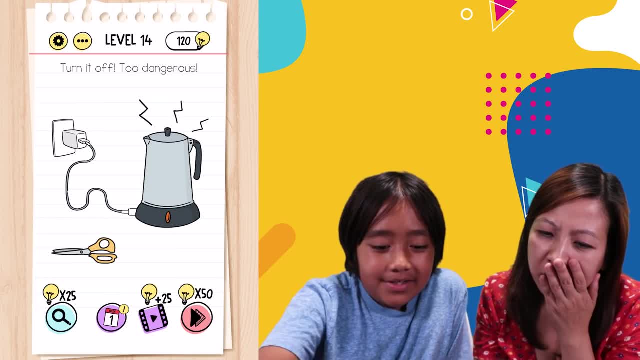 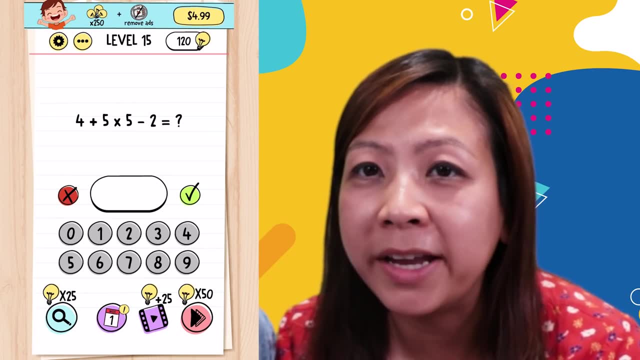 or You got it. Turn it off, Too dangerous. The off button, The button. Yay, Okay, so this is a math problem. Ryan should know he can do this. Order of operation. What do you think first, I got it, I got it. I got it. Ryan got it, I got it. 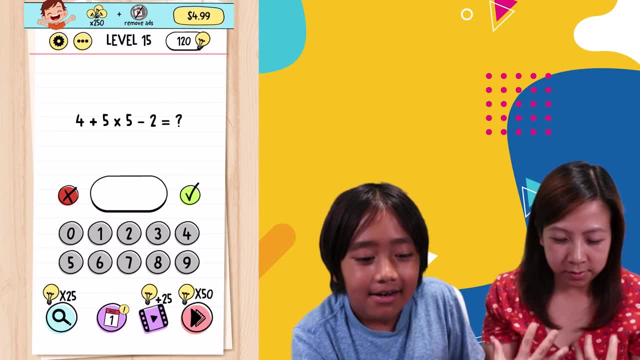 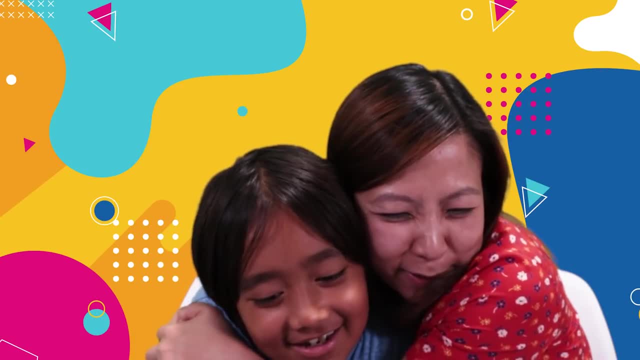 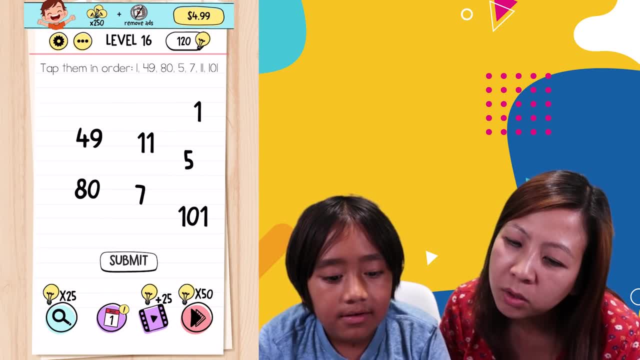 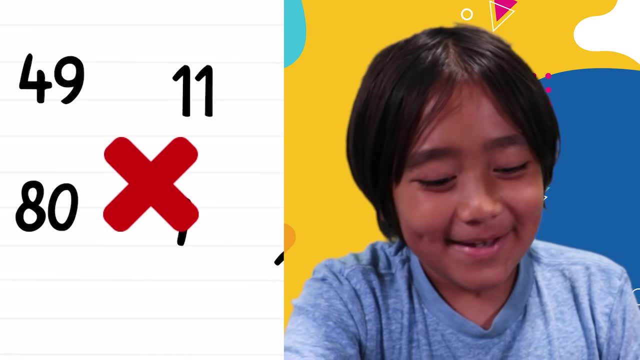 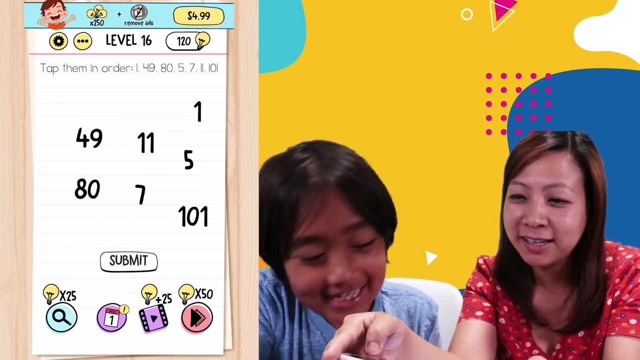 Tap them in order In order: One, Yeah, Forty-nine, Oh, I forgot the number Submit. Okay, One, Forty-nine, Eighty, No, I'm what. Yeah, Let's take a picture. Okay, Okay, take the picture. We got a picture. 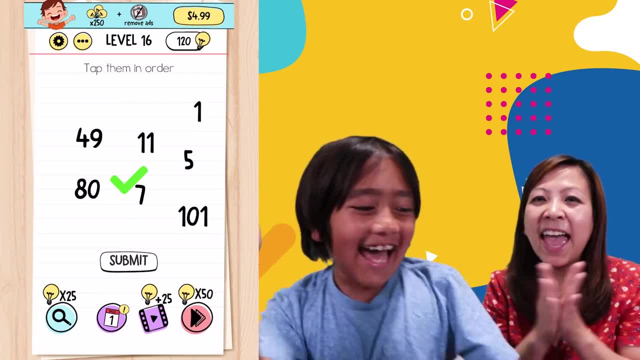 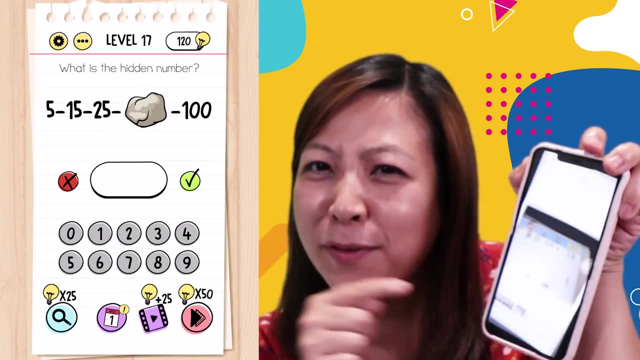 We got a picture. Yeah, Okay, Okay, Yay, That was so good. It didn't say that we couldn't do that Nice memory. You have super nice memory. Thanks, phone. What is the hidden number? Oh, 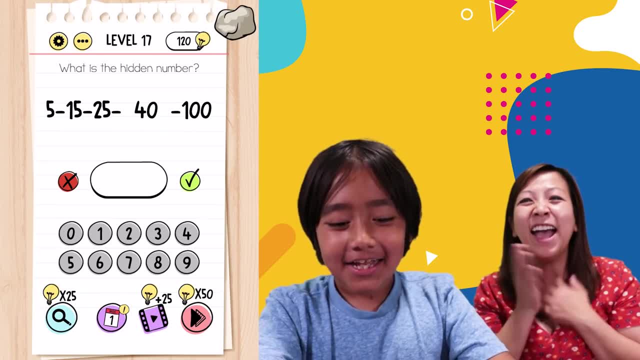 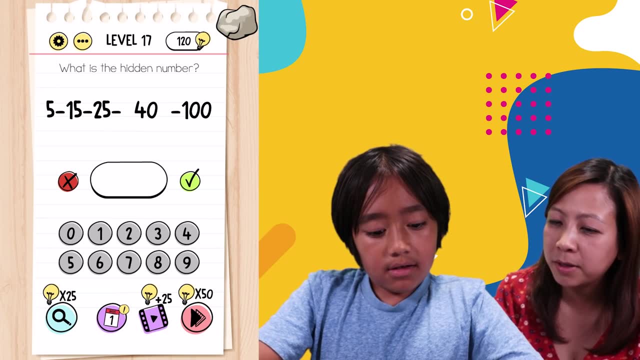 Oh, Oh, you just forgot the rock. I was gonna use my brain power. Five The hidden: it's 40, right? What is the hidden number? So you just put 40.. Oh see, Oh Nice. 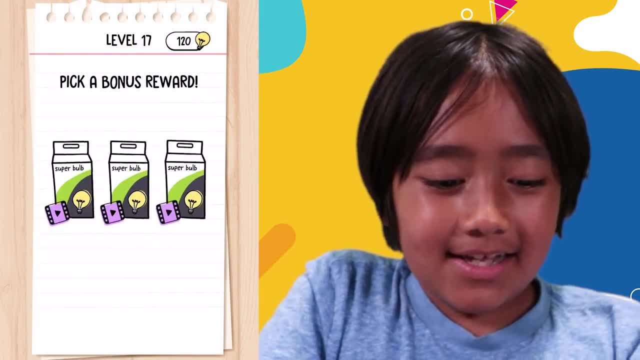 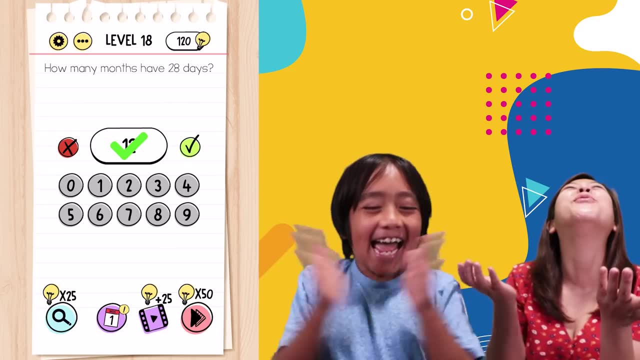 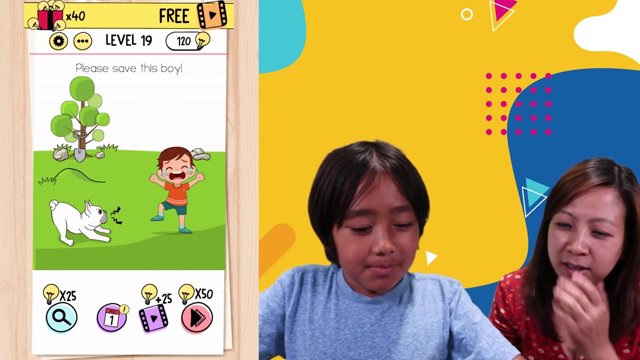 Nice, I didn't even know to lift a rock. How many months have 28 days? Only one, Only February Twelve? Oh, you're right, Everyone has 28 days. Wow, Yeah, I've heard it before. Please save this boy, How. 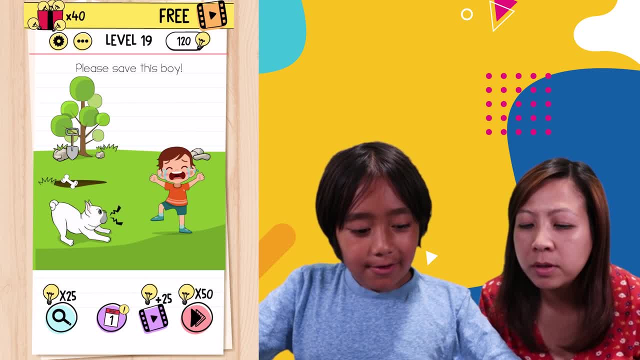 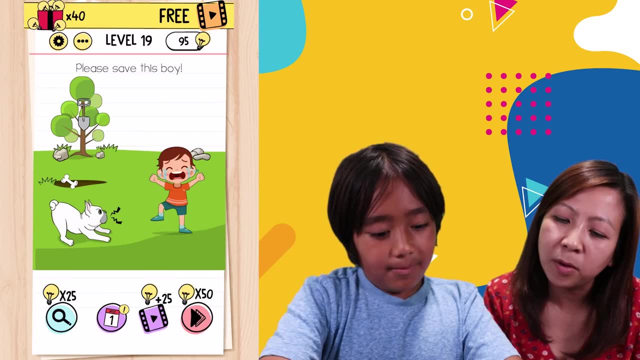 How do you save this boy? Why is there a shovel Dig? Oh, you dig the bone. Go get the bone, doggy. Go Go get the bone. We might need a hint: Dig out the bone. We did it. 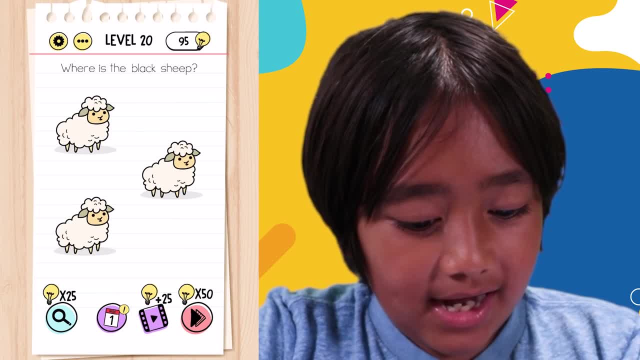 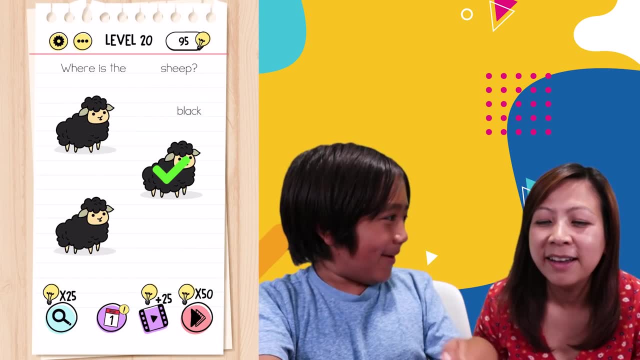 Oh, there's the bone. Yay, Where is the black sheep? Is it hidden somewhere? Oh, the word black? Oh Wait, you can. black eyes, all of them. There's an intruder in our cat party, So we maybe have to remove all the cats from here. 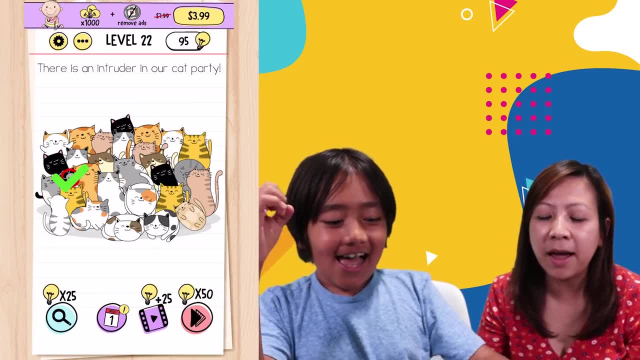 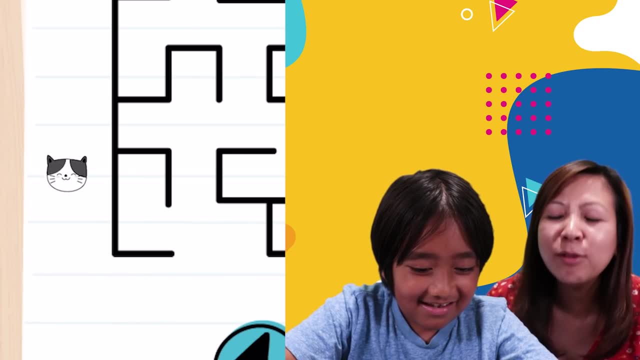 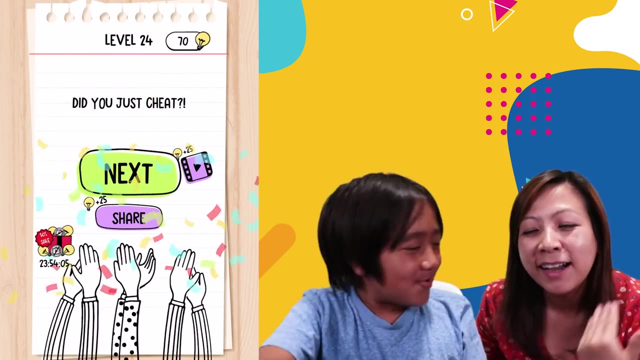 And why is that cat back there? Mouse? Oh, do you guys see that mouse? Oh, Nice, Catch the mouse, Go inside the maze. Oh, Oh, smart Ryan, I didn't even think about that. Yeah, You have to go outside the maze. 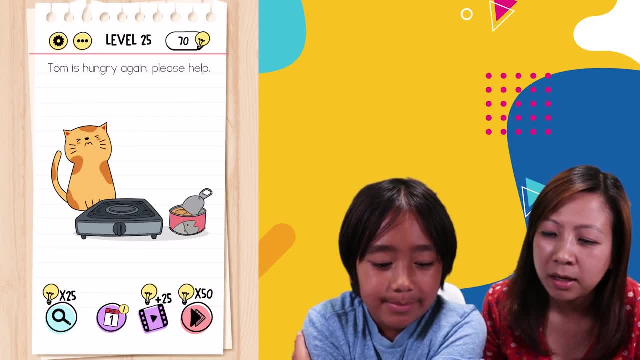 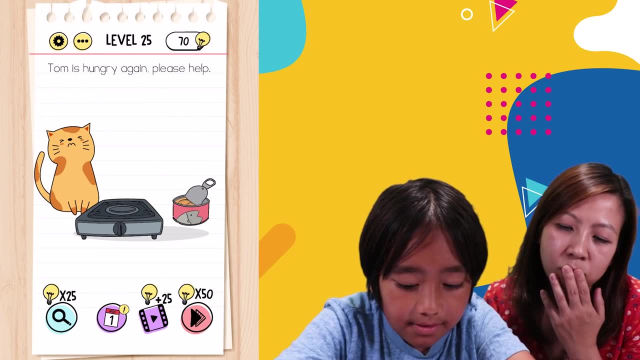 Did you just cheat? Yeah, Tom is hungry again. Please help, Where's Tom? Maybe the word Tom? Have we done that before? No, We need a hint. Nom, nom, nom. We don't want to put the cat on the stove, right. 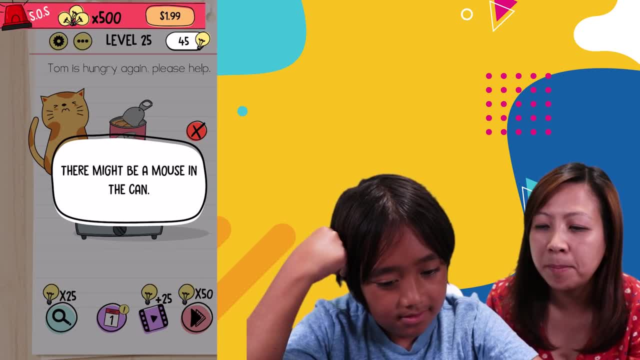 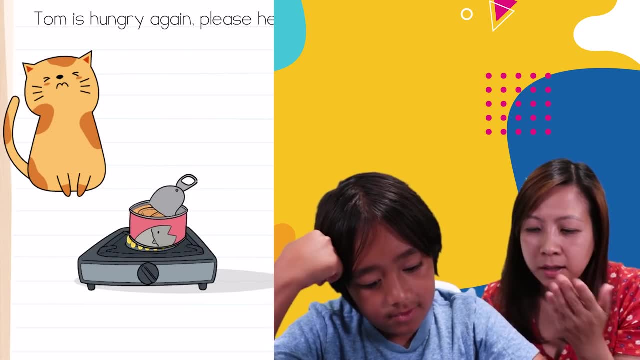 That's dangerous. I think we use a hint, guys. There may be a mouse in the can. Oh, How do we get it out? Come out mouse. Oh, maybe we put it on fire. and so the mouse gets scared and like run out. 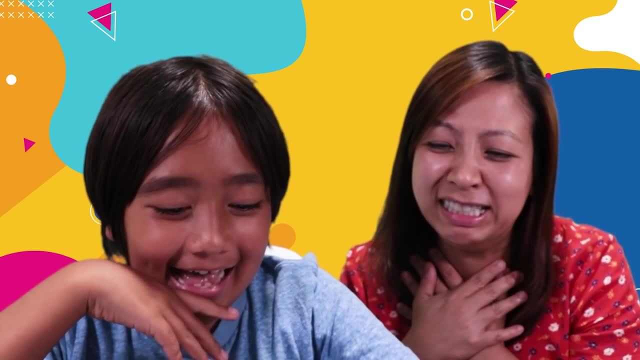 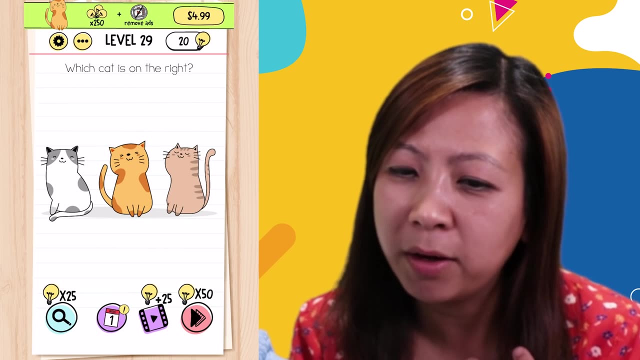 Oh, There it is. Yay, Oh, I'm so sorry, mouse. The cat is on the right. Hold on, Hold on. It's a trick question. Who's right are we talking about? Our right or their right?